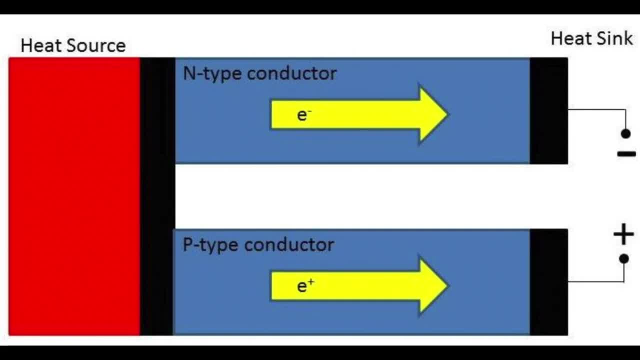 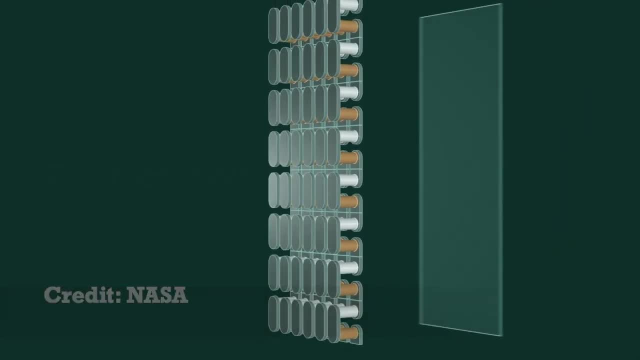 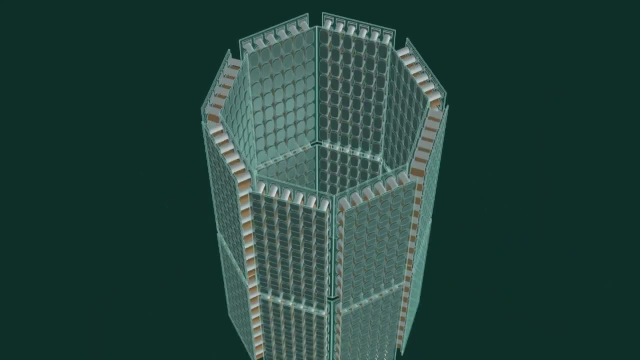 This conduction creates an electric potential or voltage between the top and bottom electrodes that can be measured. The thermocouple, when combined with hundreds of others, just like it, can be shaped and stacked to form a hollow tube. The heat source would be placed inside the tube, with the outside of the tube being colder. 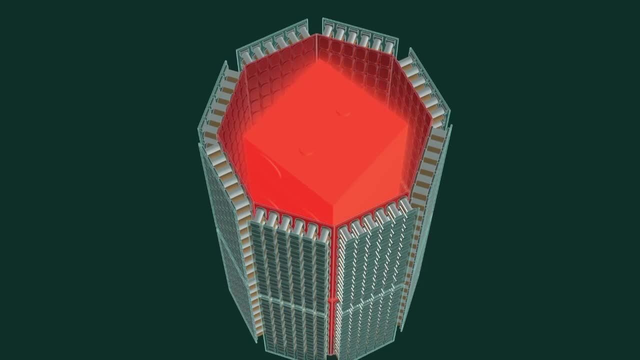 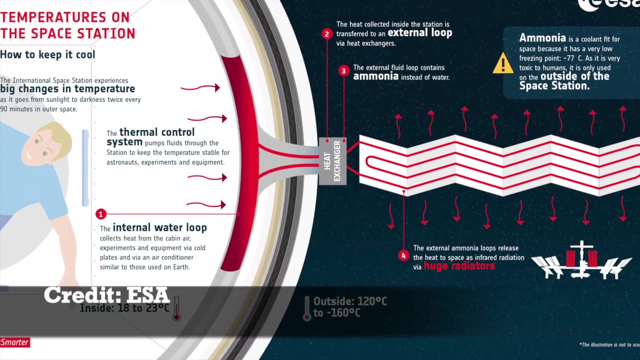 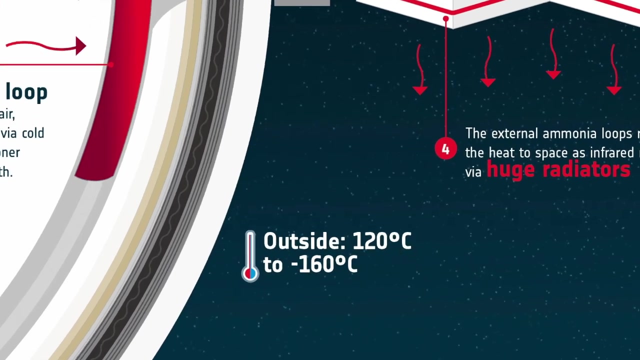 The temperature gradient can then be exploited to maximize the difference between hot and cold ends, producing more electricity. In deep space. we can maximize the cold side to well below 150 degrees centigrade Nearer to the sun. however, surface heating does raise the temperature drastically, limiting 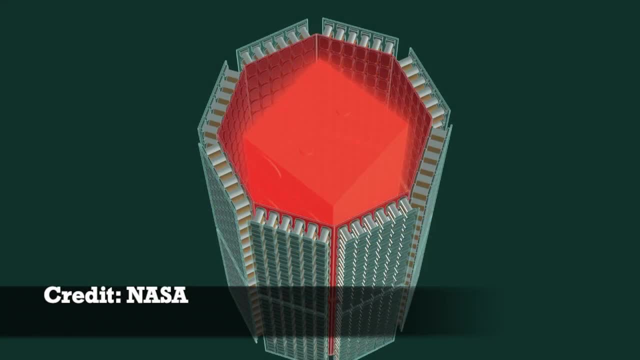 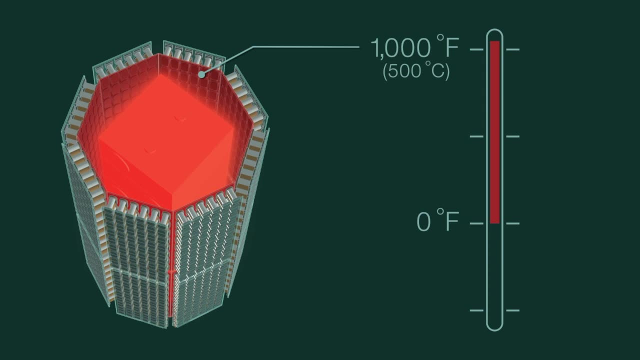 the thermocouple's efficiency. Using a nuclear heating source like plutonium, the hot end of the thermocouple can be more than 500 degrees centigrade. This, when compared to the much colder temperature of space, creates a large difference. thus, 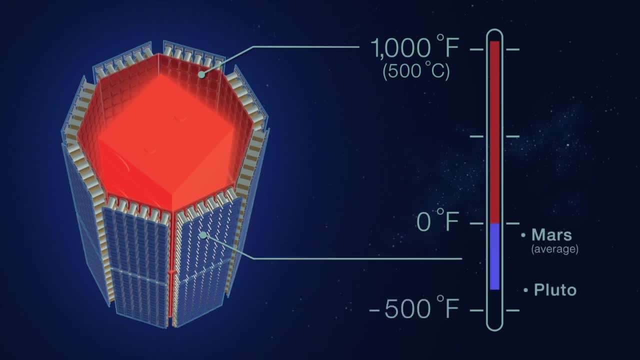 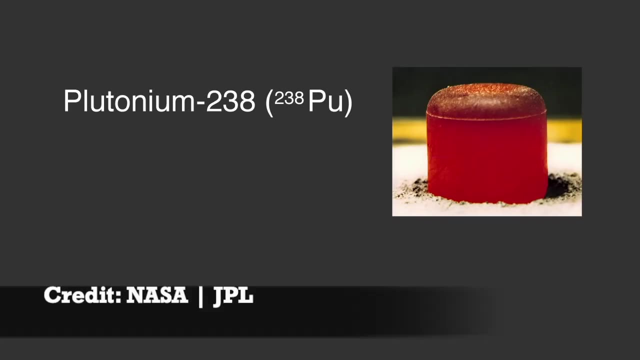 enabling a larger amount of electricity to be produced. Let's take a closer view at this nuclear heating source and how it was designed with safety in mind, Specifically used for radioisotope power systems. plutonium-238 is an alpha emitter, meaning 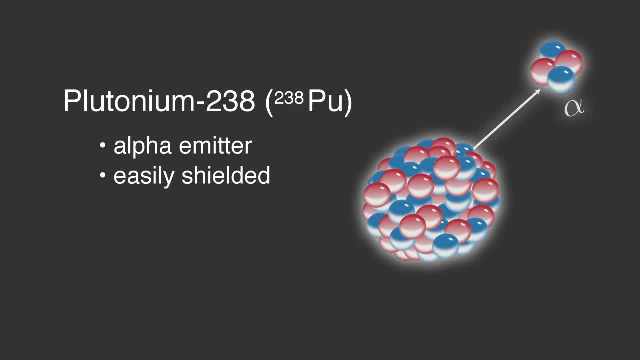 its radioactive decay or heating is due to alpha particles. These alpha particles are easily shielded, providing easy heat collection and safety to humans near it. It's only harmful to humans if it is inhaled or ingested. Making it safer still, the RPS uses plutonium-238 dioxide. 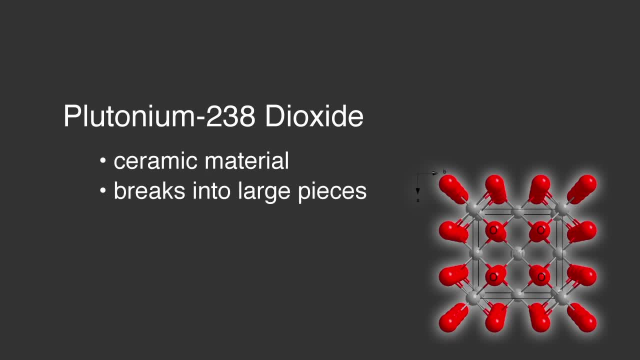 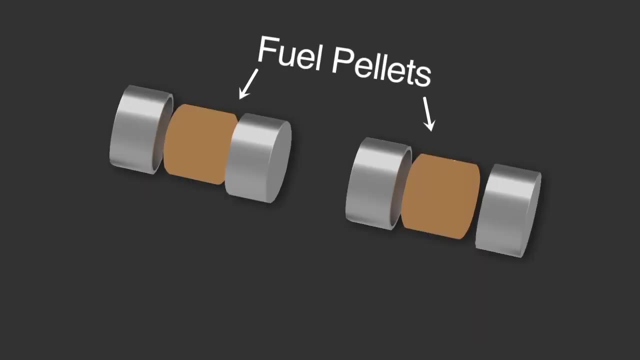 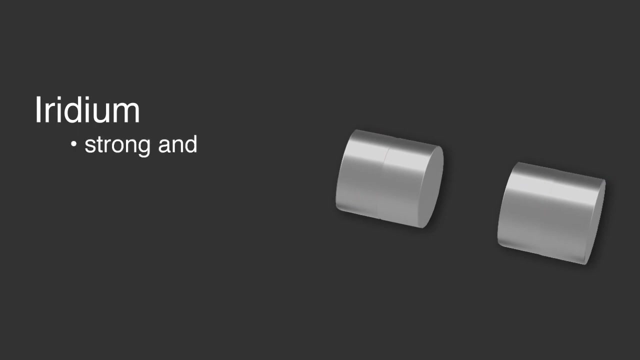 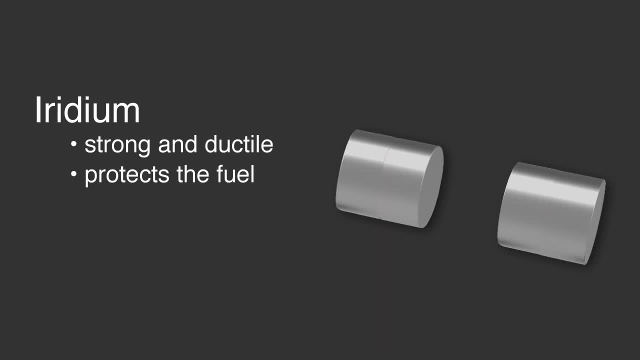 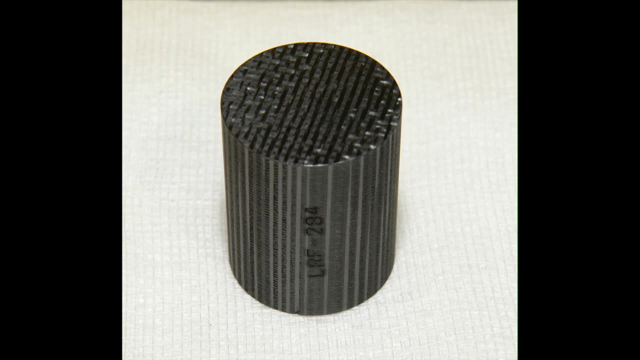 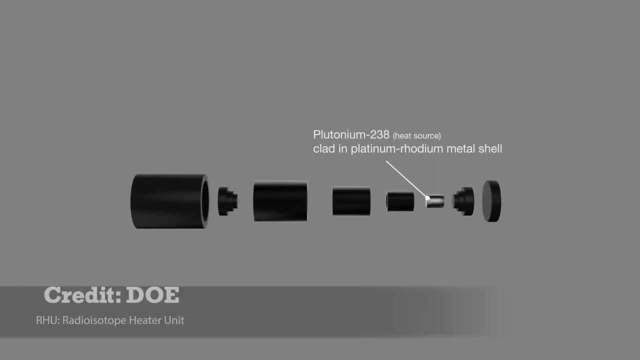 This means that the emitter will keep your end of the thermocouple from getting damaged, and material compatibility. The encased fuel pellet is the perfect form factor for a radioisotope heater unit, or RHU, delivering heat to systems in the coldest parts of space. Let's take a look at the RHU: The plutonium fuel is encased. 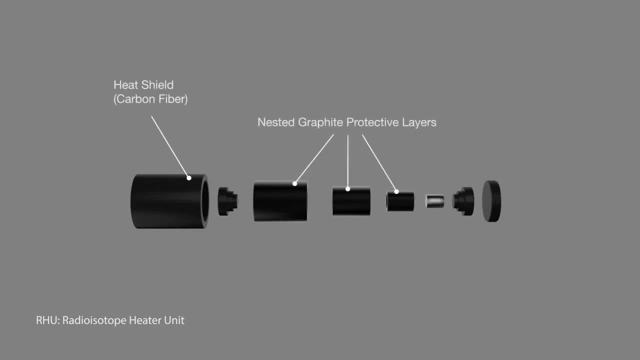 in the iridium material. at its center, The pellet is nested in three layers of graphite, each slightly larger in size. Finally, the whole thing is encapsulated in a carbon fiber shell for physical protection. Each RHU can then produce up to one watt of heat for the spacecraft's systems in deep space. Several NASA. 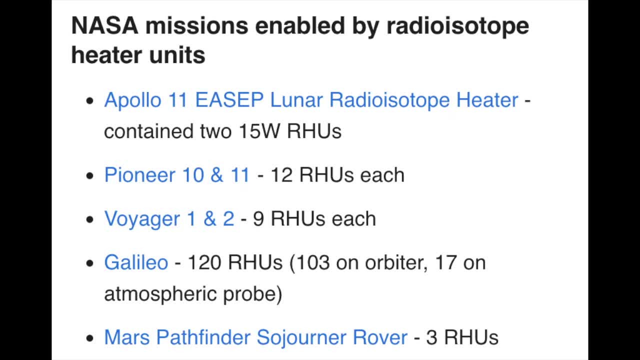 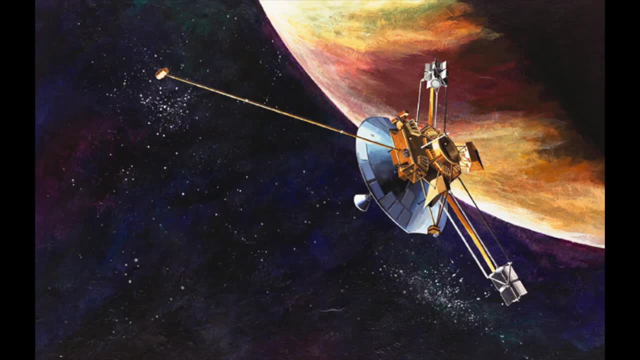 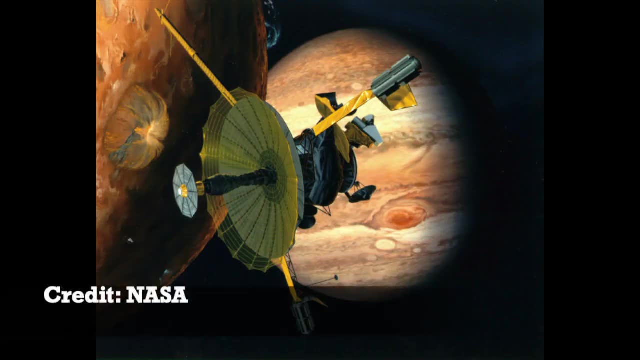 missions have utilized RHUs in various quantities and heat outputs. Pioneer 10 and 11 each had 12 RHUs on Jupiter and Saturn flybys Voyager 1 and 2 have taken 9 RHUs each around the outer solar system's planets, And Galileo used 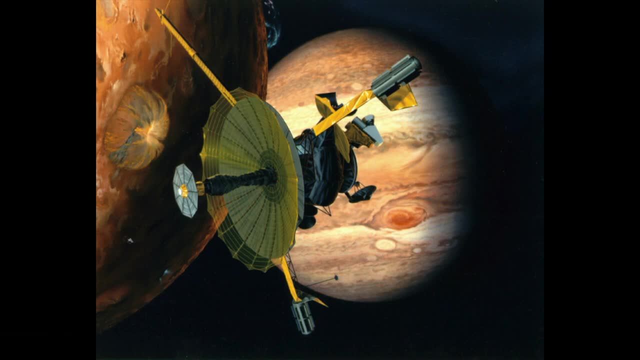 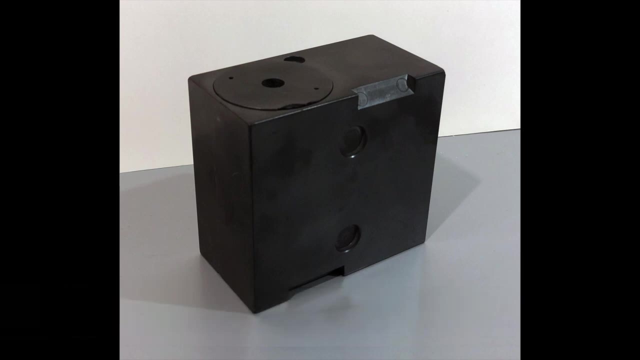 120 RHUs in its orbital study of Jupiter and its moons, Using similar fuel pellets to the RHU. the General Purpose Heat Source Module, or GPHS, is the essential building block for the radioisotope generators. Each GPHS weighs. 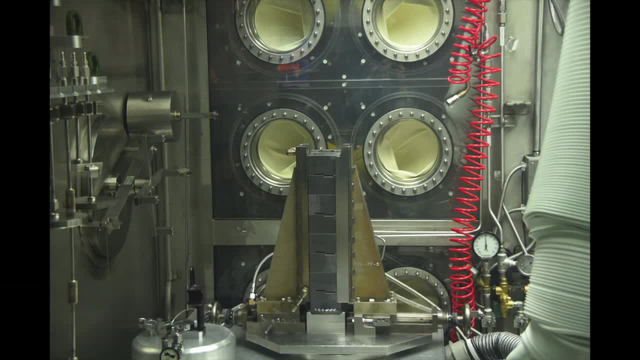 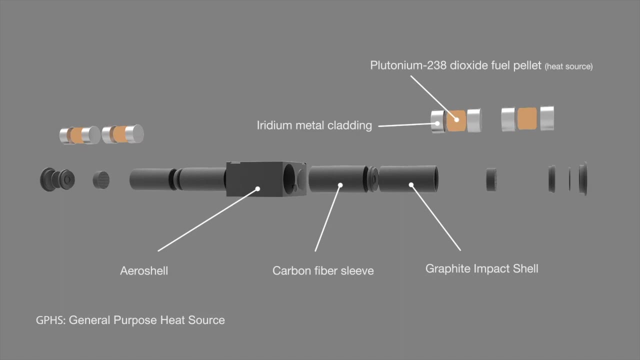 approximately 1.5 kilograms. They're designed to produce 250 watts of heat and can be used individually or stacked together to increase the heat generated. Exploded View: lets assemble a GPHS. Internally, each has two plutonium fuel pellets clad in. 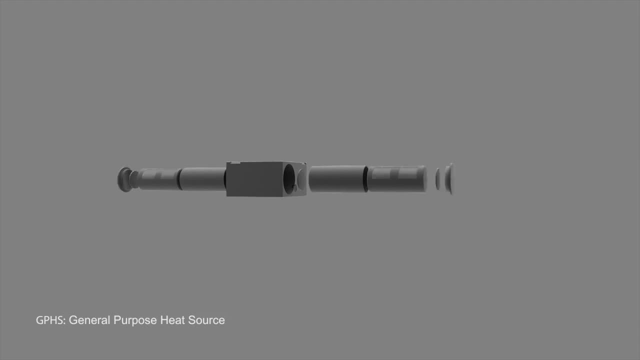 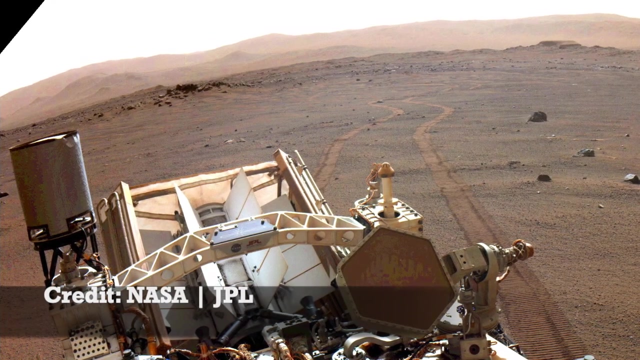 iridium. Those pellets each have a graphite impact shell and multiple carbon fiber sleeves. Both, however, are housed in a single aeroshell to protect against re-entry in the event of a failed mission launch. We've now covered each component that would make up a radioisotope. 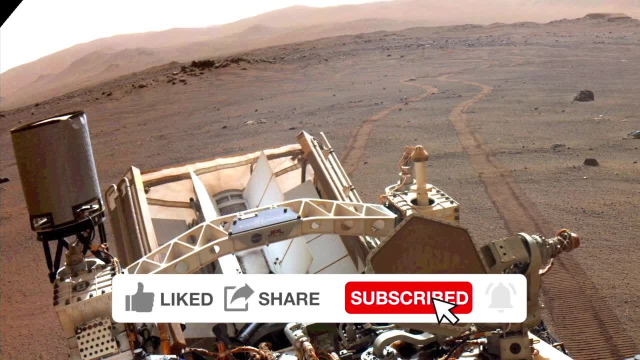 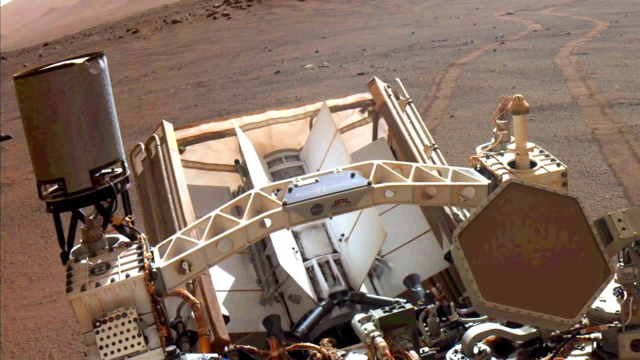 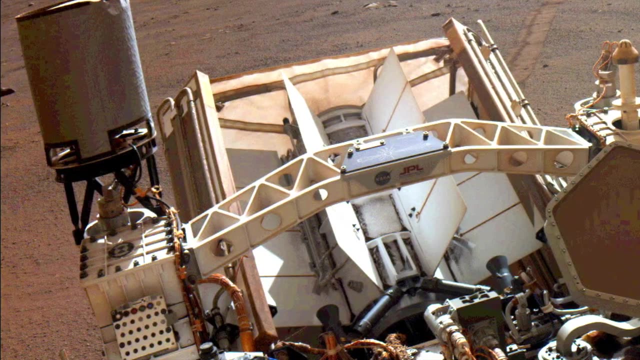 thermal generator Together, designed for maximum power output and safety. they make up the radioisotope thermal generator. GPHS is the main power source in so many of our probes. The latest certified RTG is the Multi-Mission Radioisotope Thermal Generator, or MMRTG, seen here on the Perseverance rover. 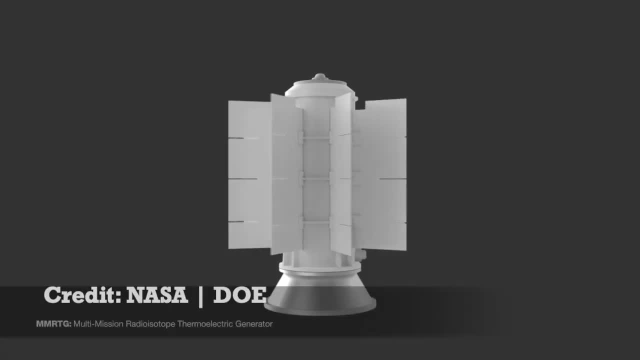 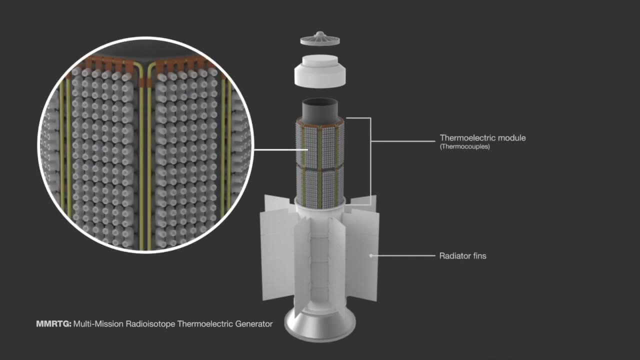 An MMRTG generates about 110 watts of electrical power at launch, While the outer casing holds radiator fins to help with excess heating. the thermocouple module is made up of 768 thermocouples At its core, the GPHS module we discussed.